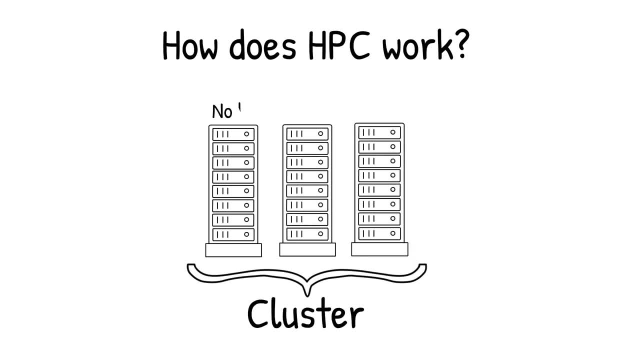 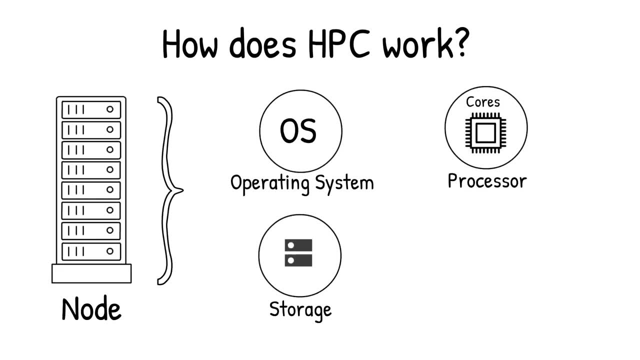 You can think of a high performance computing system as a high performance computer that is able to perform high performance tasks. It has a group of computers called cluster and each computer in a cluster is called a node. Each unit in the cluster has an operating system, a processor with multiple cores. 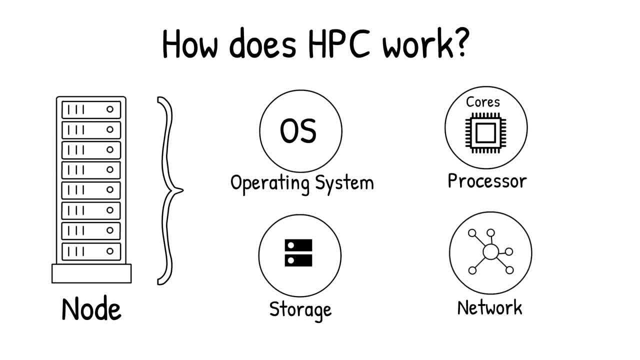 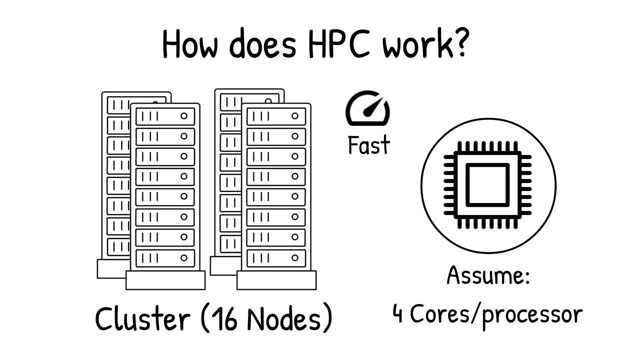 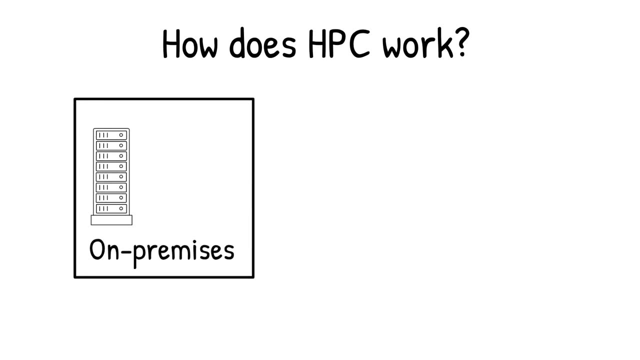 storage and networking capabilities for the units to talk to each other. A small cluster, for example, can have 16 nodes with 64 cores, which is four cores per processor, helping you solve a problem much faster. A supercomputer is a much larger variation of this HPC job that would run across. 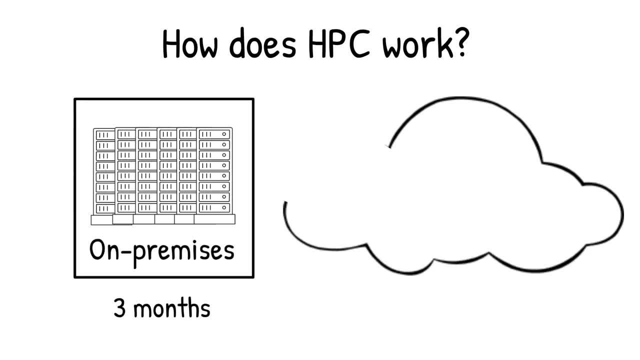 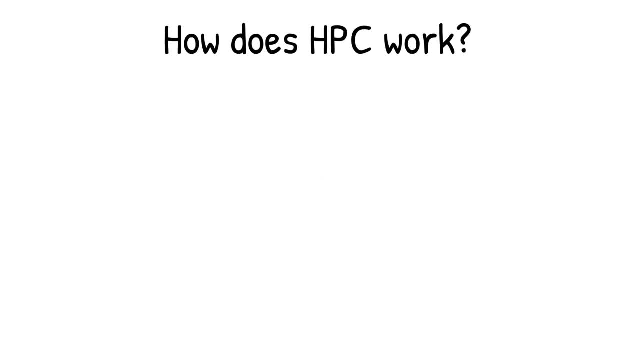 an on-premises cluster for three months could run across 125,000 cores in 16 hours in the cloud at little or no incremental cost, And by augmenting your HPC environment with Google Cloud you gain economies of scale with access to the largest compute and storage hardware. 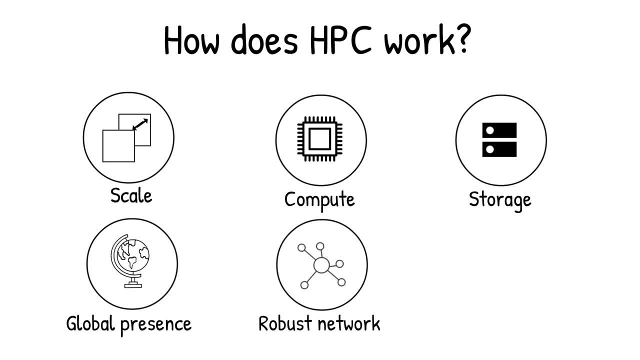 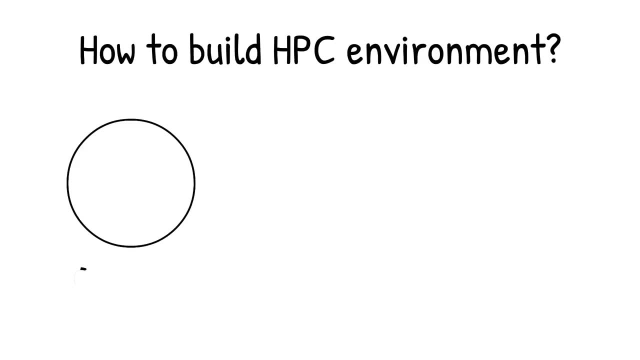 global presence, robust networking and intelligent automated management capabilities on the cleanest cloud. Now how to build HPC environment on Google Cloud. Compute storage and networking are the building blocks of high performance computing. Compute Engine provides customizable virtual machines running in Google Cloud. 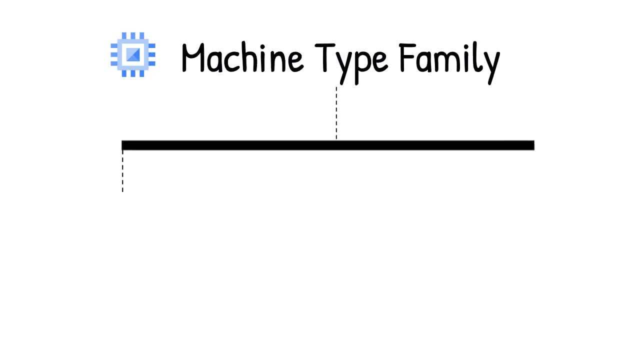 You can scale up and down as needed and choose from a range of machine types for your workloads. We recommend the compute optimized C2 machines for most high performance computing applications, but you can also select the general purpose- N1,, N2, or N2D for applications requiring larger memory. 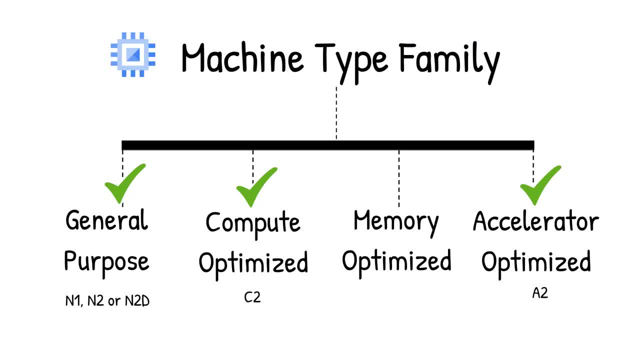 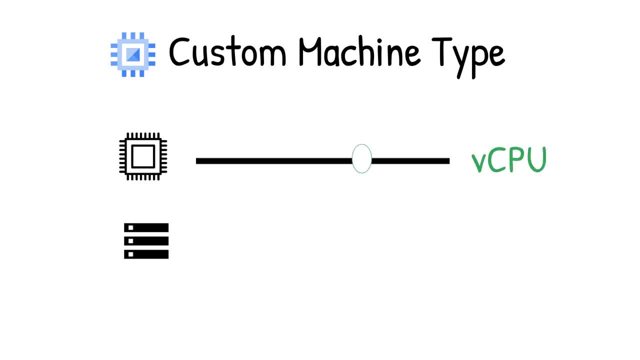 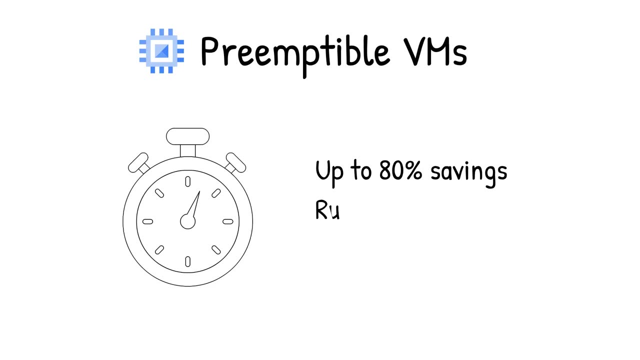 sizes For very specific requirements. you can choose custom machine types with the exact number of cores and memory to match your workload requirements and get the best performance per dollar. You could also use cost-effective preemptible VMs, which are short-lived compute instances. 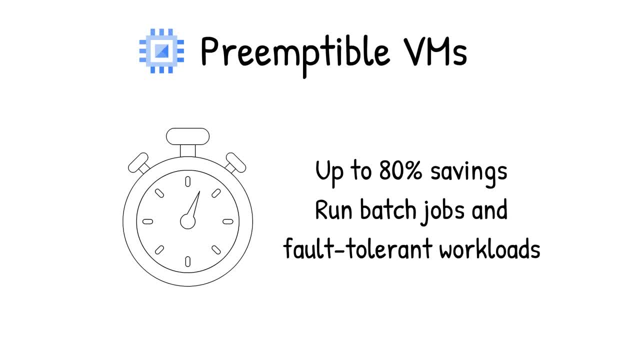 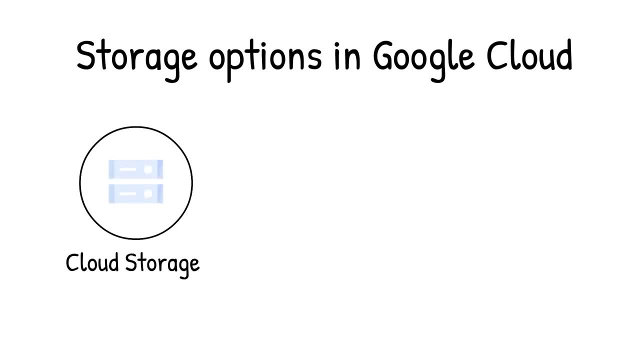 suitable for batch jobs and fault-tolerant workloads. Now the underlying storage system is critical to the performance of many HPC applications. You have a lot of storage options in Google Cloud. Cloud Storage is a highly scalable object store to store any amount of data. 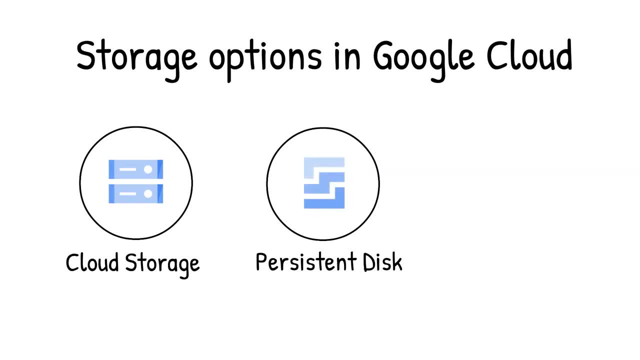 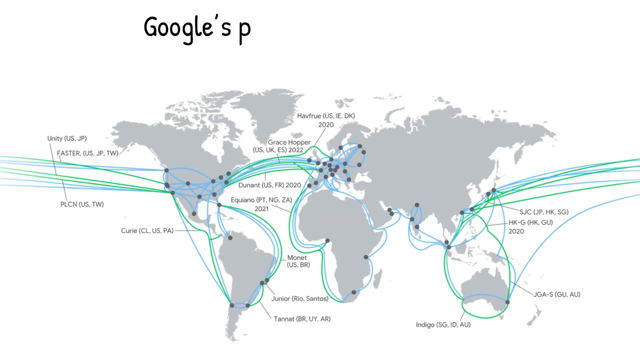 Persistent disk is durable and high-performance block storage for your VM instances. File Store High Scale is a high-performance scale-out file system that makes it easy to mount file shares on Compute Engine VMs. Google's privately managed global network infrastructure ensures that your data and 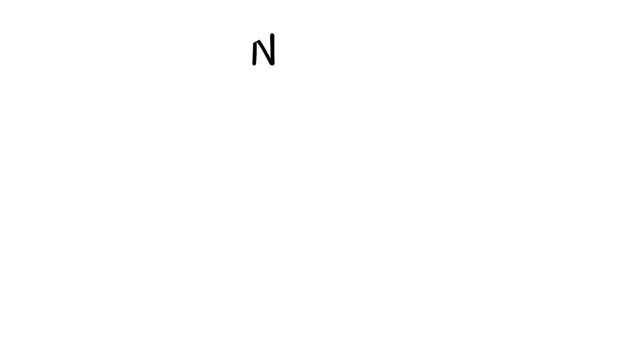 applications are the least-discorded and most reliable source of data. Virtual Private Cloud VPC networks are available to enable connectivity from your Compute Engine VM instances and configure firewalls for your applications. With Placement Policies, you can control the placement of your VMs in our data centers. 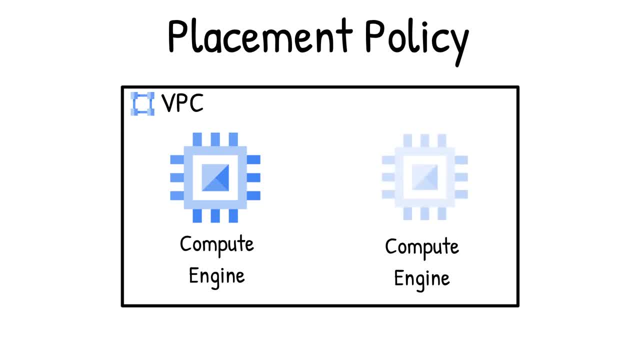 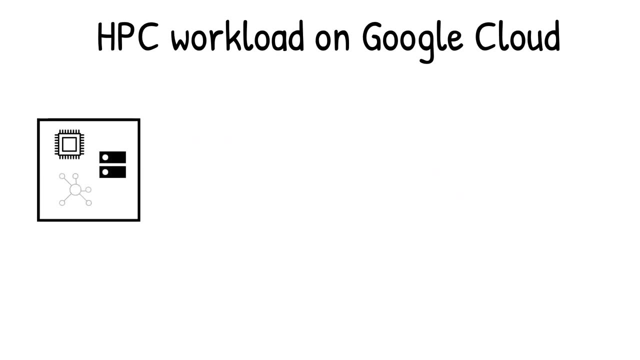 Compact Placement Policy provides low latency between nodes by placing instances close together within the same network infrastructure to speed communications between nodes. Now let's put it all together for your HPC workload on Google Cloud. First, determine the compute, storage and networking requirements for your HPC code. 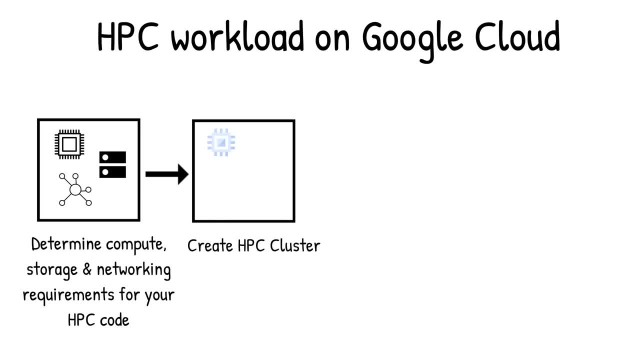 Then create your HPC cluster using Compute Engine instances connected to the storage of your choice. Additionally, Google Cloud supports several job schedulers, making it easy for you to start auto-scale VMs to meet job requirements or spin down a cluster when a job is complete. 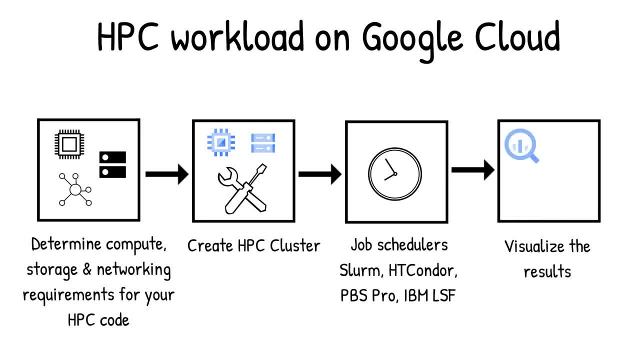 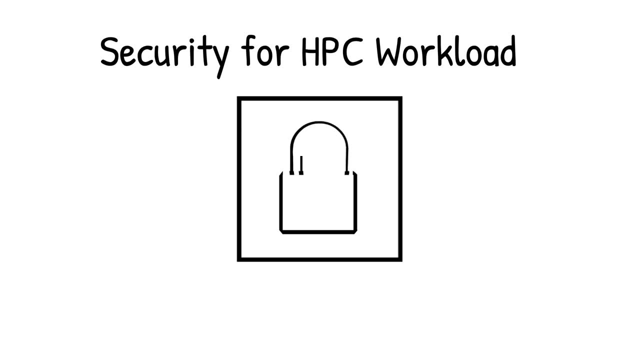 helping save cost. Then visualize your result in BigQuery or AI Platform for post-processing From there, just monitor the performance and change the cluster as needed. Security is important for any HPC workload. Google Cloud's Secure-by-Design infrastructure protects your data. 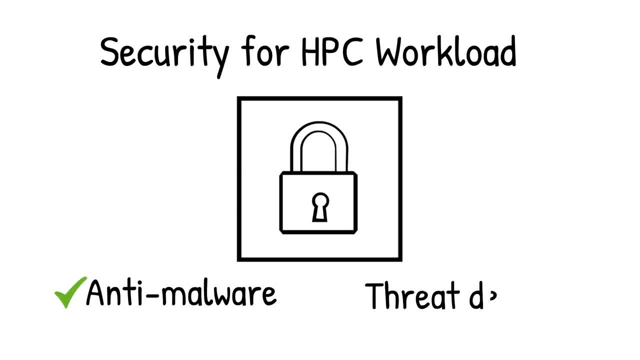 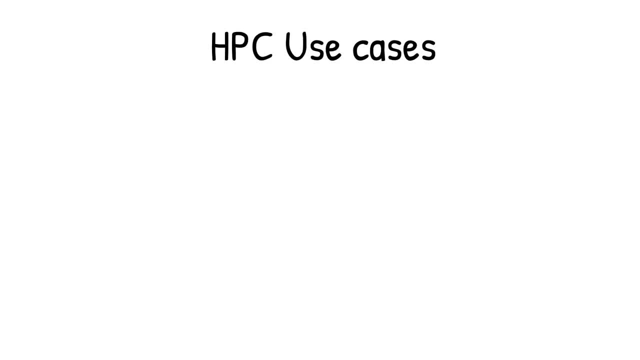 applications and users with advanced anti-malware and threat detection. High-performance computing drives research, development and innovation in many industries, from rendering the visual effects in the lab to the cloud, The latest blockbuster movie- to sequencing the human genome to cure diseases. 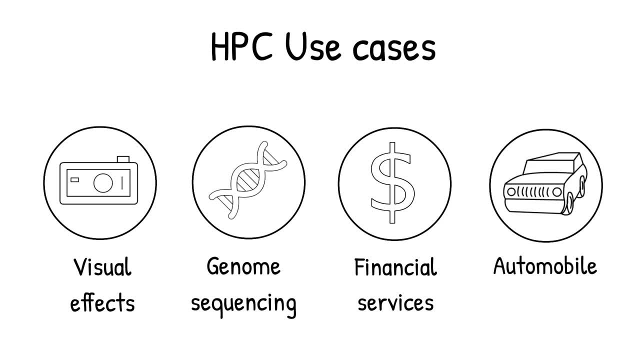 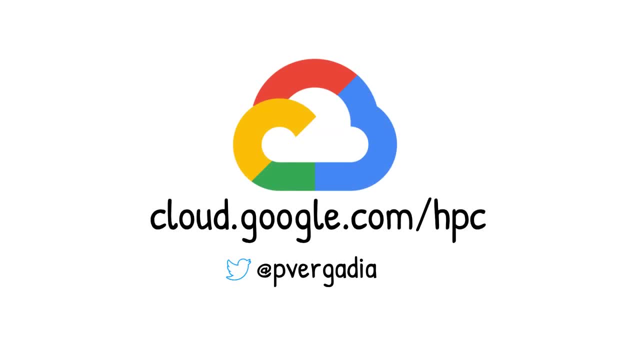 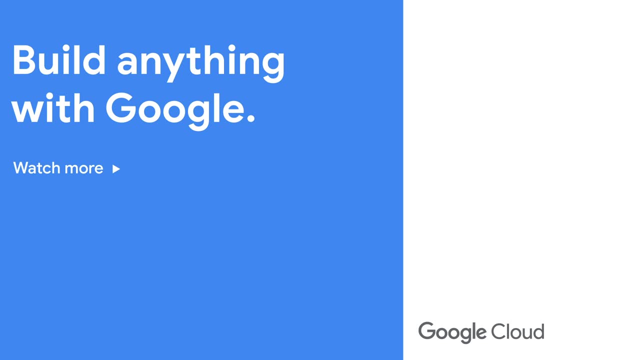 to risk analysis in financial services or even to design the next generation of cars. If this has piqued your interest, visit cloudgooglecom to learn more and get started wwwcloudgooglecom.